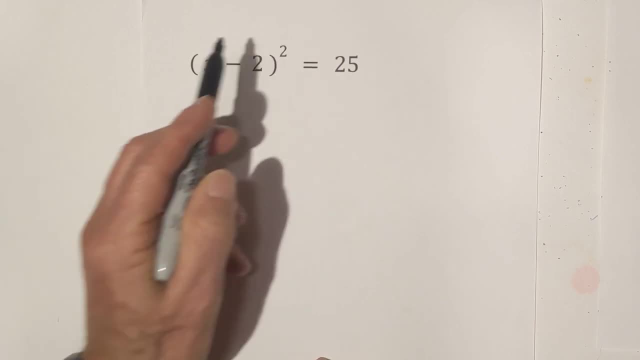 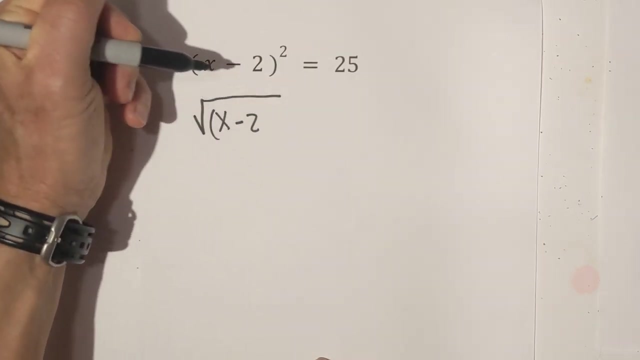 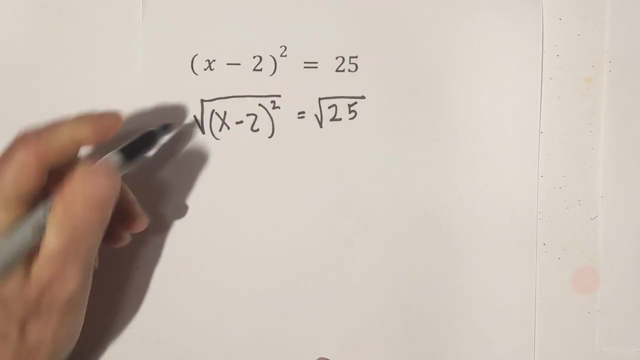 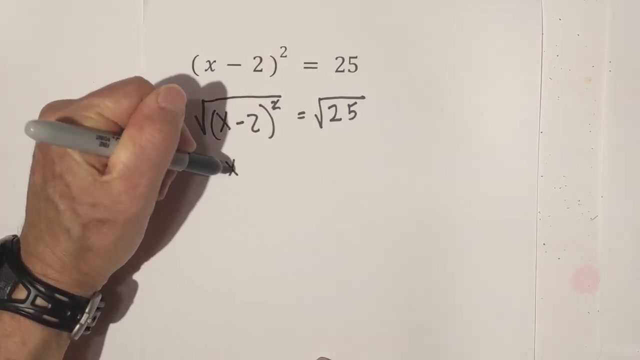 First, what we need to do is get rid of the square, And so, in order to do that, we're going to find the square root of both sides, Okay, and the square root of 25.. So, whenever we go with this, the square root will be this cancels, so it will be x minus 2 equals, and I know the square root of 25 is 5.. 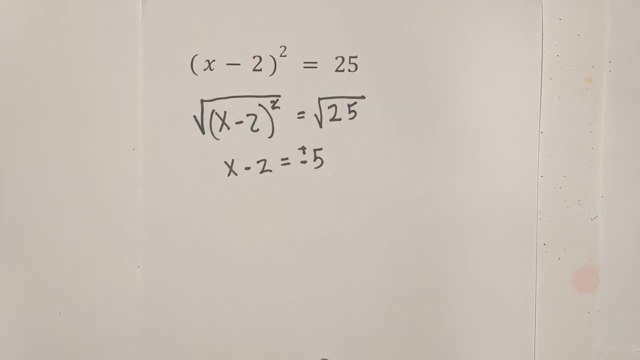 But it is plus or negative 5.. So now what we will do is we will solve it for both a positive 5 and a negative 5.. So what we're going to do is we're going to add 2.. And so let's work the first one over here. We have x minus 2 equals 5.. So we're going to add 2 to both sides. Okay. 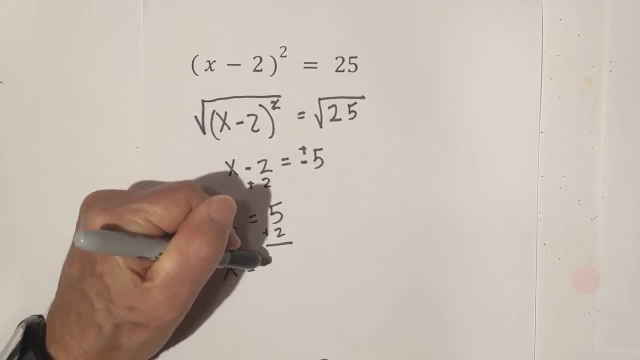 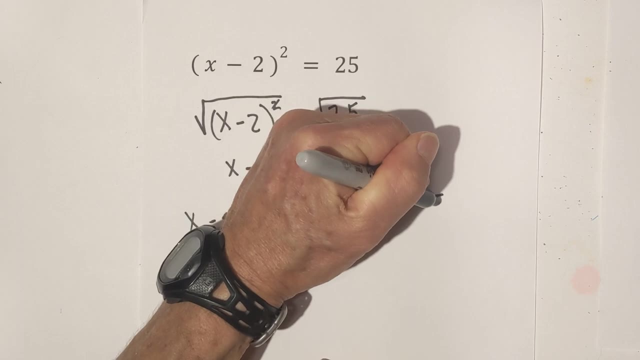 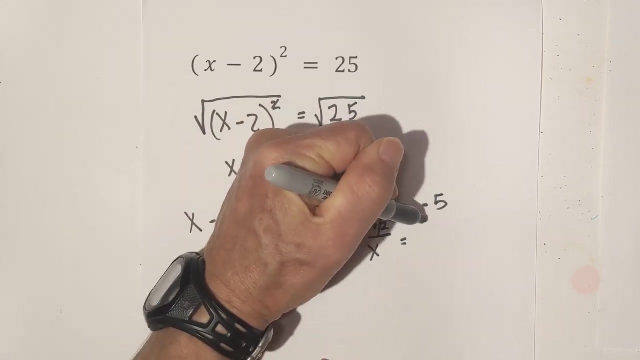 And so these cancel, so it becomes x equals 7. And then we have x minus 2 equals a negative 5. And so we add 2. And so we bring down the x equals. we add 2 here. That is a negative 3.. 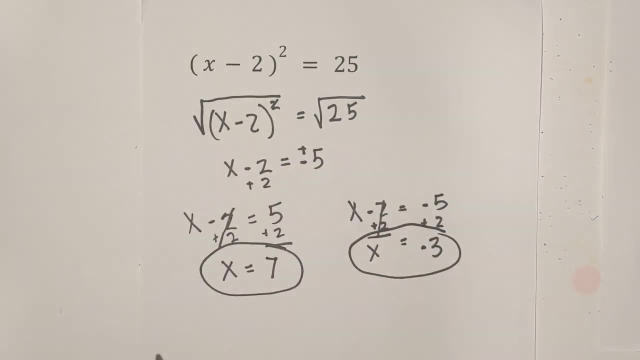 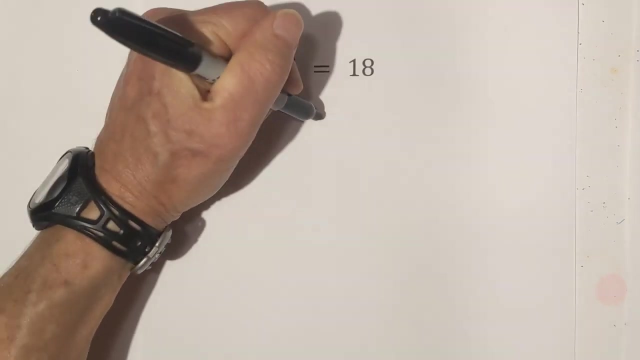 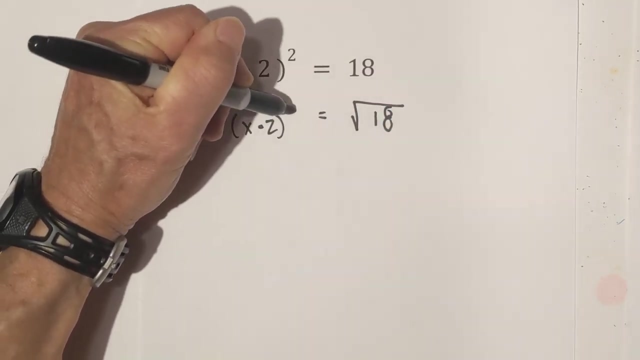 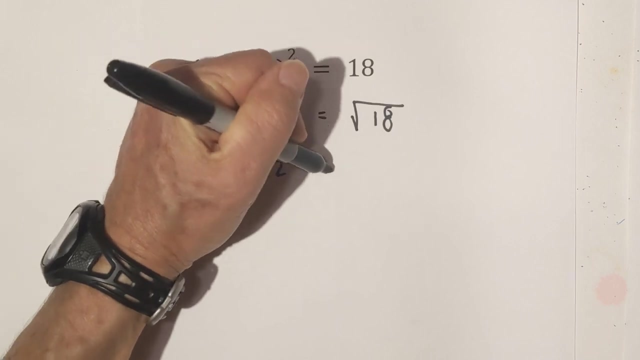 So there are your two solutions. Let's work another example Now. in this example, 18 is not a perfect square, So we'll have to add a couple steps. So we first need to get rid of the square, And so we're going to take the square root of both sides. Okay, so we have x minus 2 squared. Okay, the square root of this will be x minus 2 equals. Now let's see what we can do with this square root. We can take some numbers out. 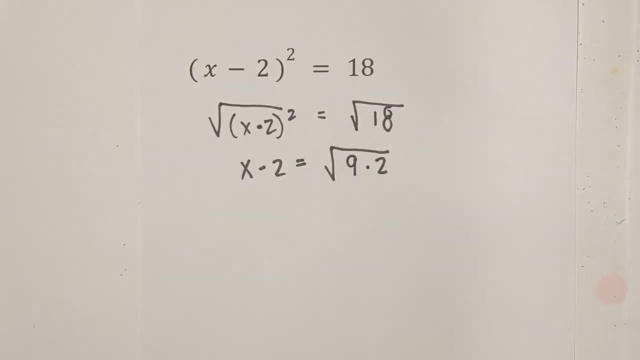 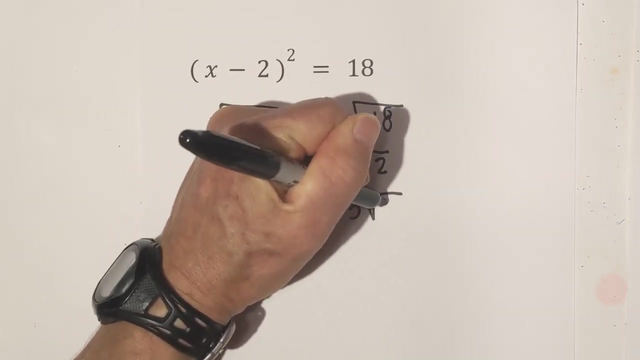 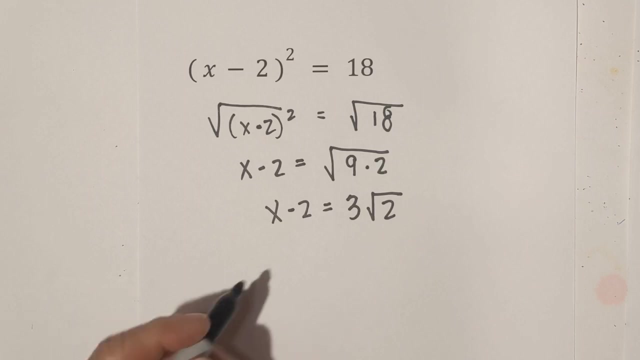 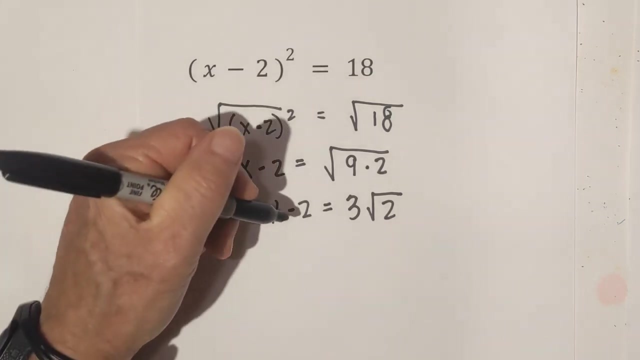 9 times 2 equals 18.. The 9 is a perfect square, So I can take a 3 out. Okay, so now we have x minus 2.. Okay, equals 3, square root 2.. So now what I need to do is get x by itself, So I'm going to add 2. And once again, this is a plus or minus. 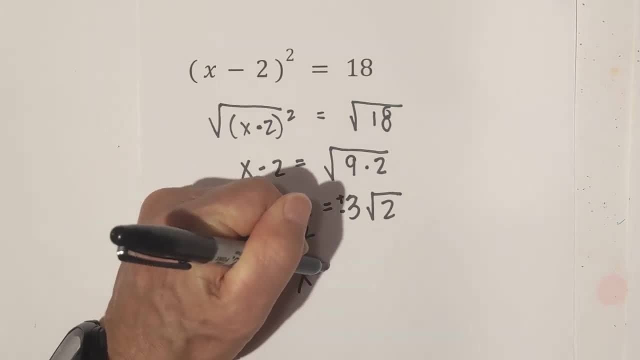 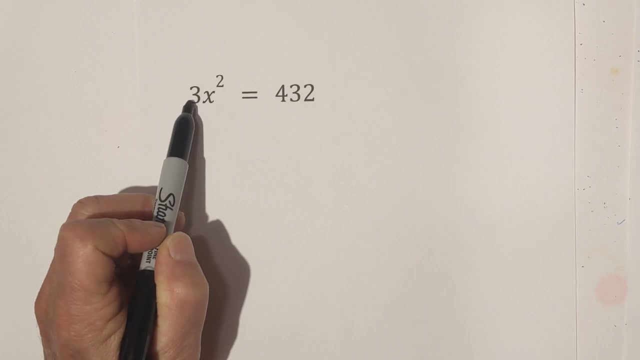 Minus. So it will become x equals 2 plus or minus 3 square root 2.. Okay, so there's your solution. Let's work two more examples you may encounter. Okay with this example, remember the square that the is attached to the x, not the 3. So we need to get x squared by itself. 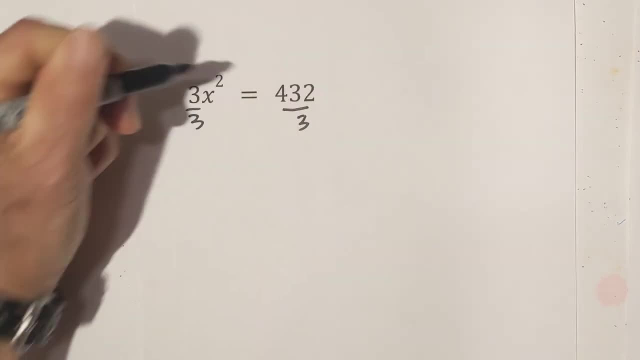 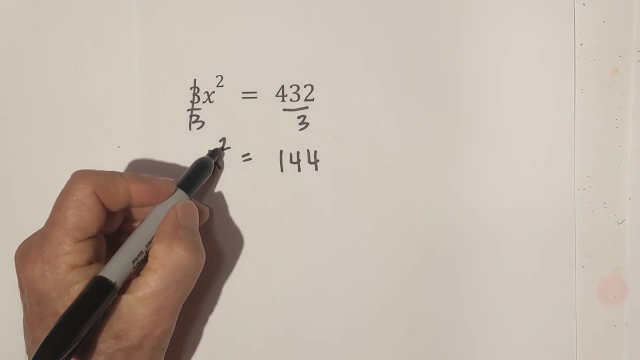 So we're going to divide both sides sides first by 3. these cancel. so we have x squared equals 432 divided by 3 is 144. okay, now what we do is we need to get rid of the square by taking the square root. okay, and excuse me, that square root of x squared and that becomes x equals and the square root of. 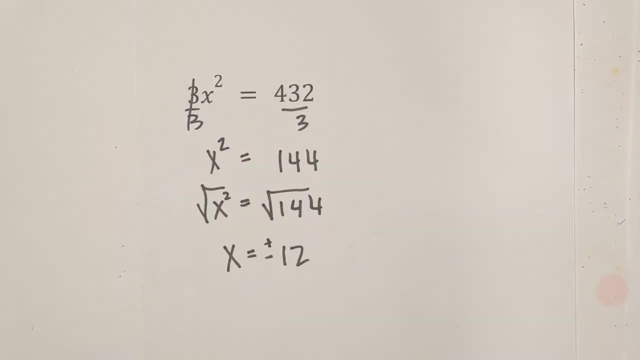 144 is 12 and remember it's plus or minus. okay, i thought that one, that one, was pretty straightforward, okay. one final example: okay, this example has- okay, this one has a little bit of everything in it. so let's get rid of the square root of x squared and we're going to take the square root of x squared. 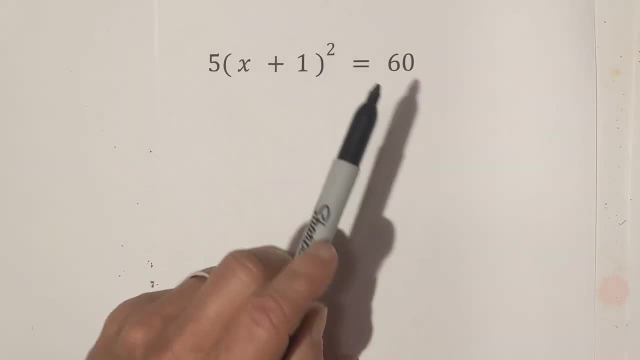 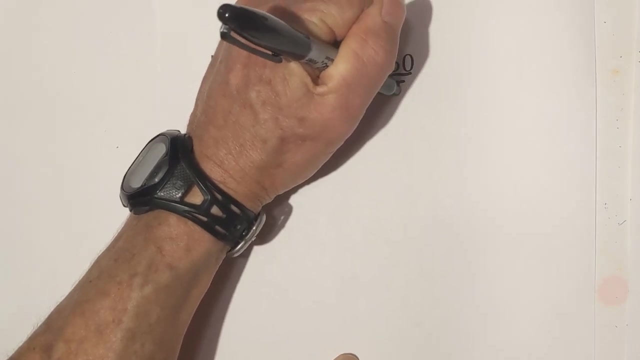 get started first. we want to get x by itself. the square root is attached to x plus 1, so we need to get rid of the 5. so I'm going to divide both sides by 5. these cancels okay. so we have x plus 1. 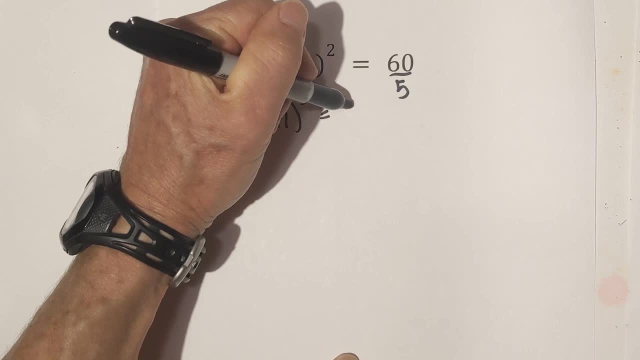 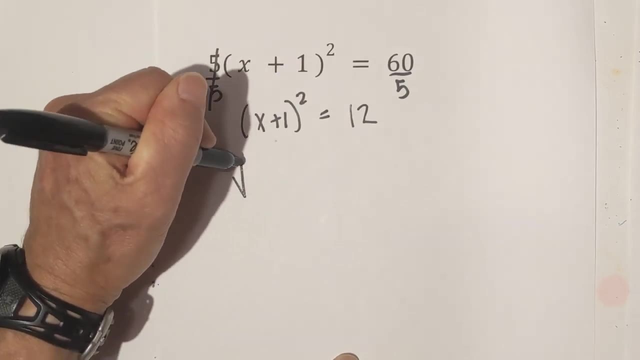 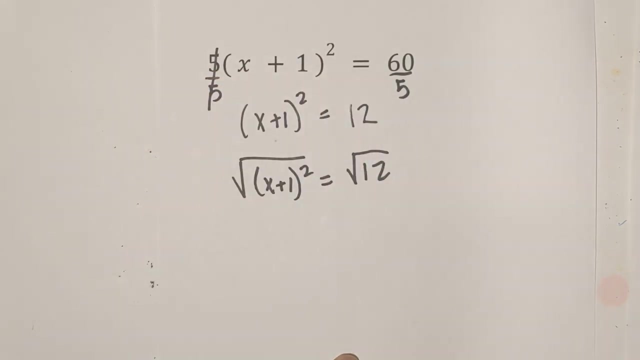 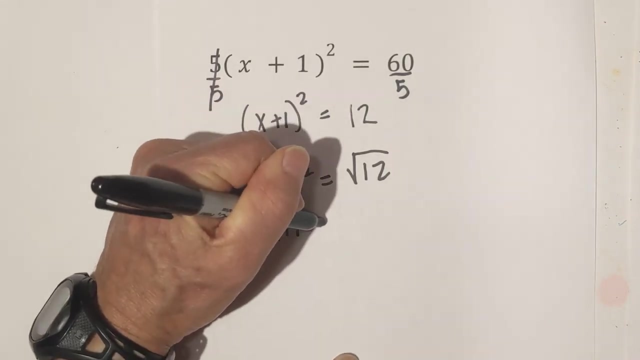 squared equals 60 divided by 5 is 12. okay, now, what do we do next? let's get rid of this square by taking the square root. so we have x plus 1 squared equals the square root of 12. okay, now, this now becomes: we take the square root of this is x plus 1 equals and the square root of 12 it's. 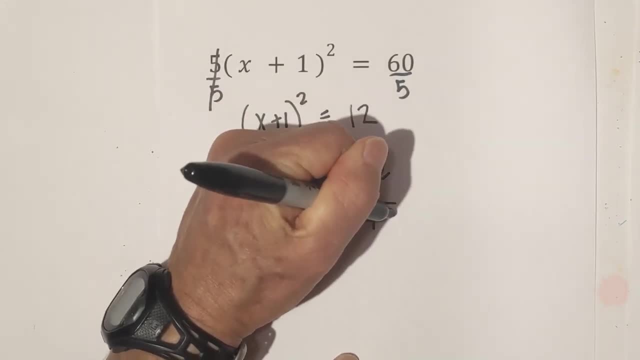 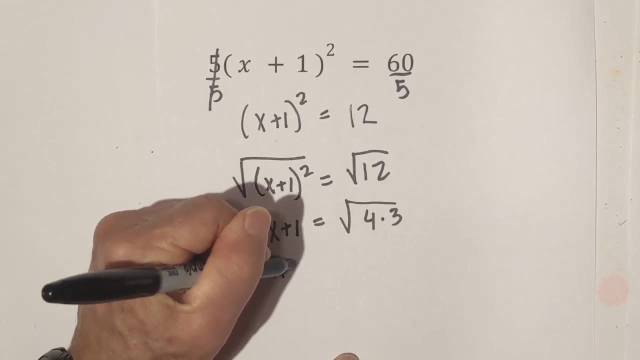 not a perfect square, but we can go 4 times 3, so 4 is a perfect square, so we can take that out. so we have x plus 1 equals square root of 4, 4, 2, square root 3. now what do we do here? but remember, it's plus or minus, well we?